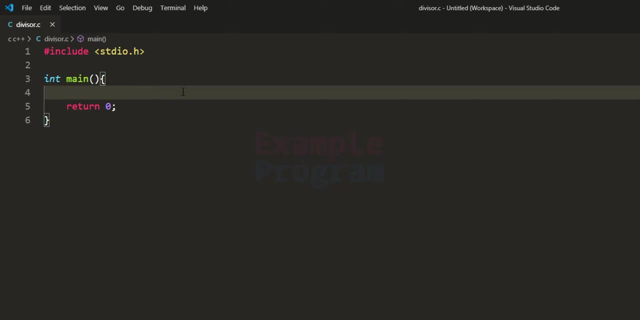 use it for a natural number, So we will display all the divisors for a natural number entered by the user. So here I have included the stdioh header file so that we can use the functions like printf and scanf, and then I have returned this main function, which is the entry point of our 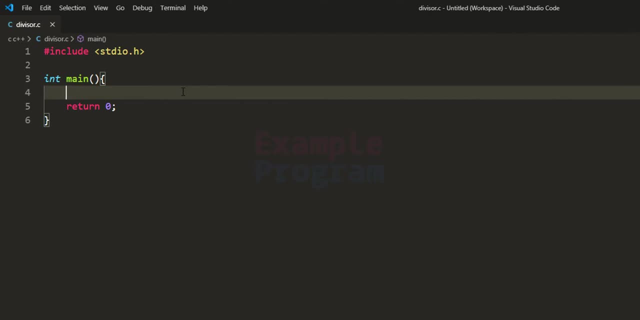 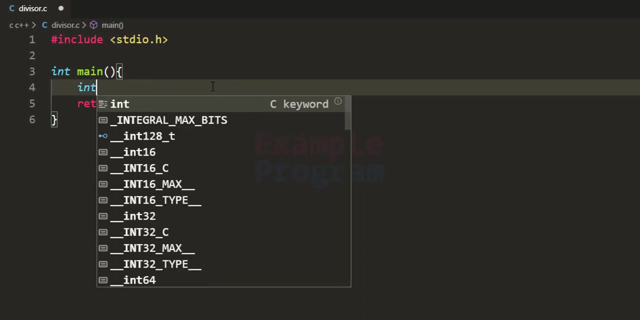 program from our perspective. So here the first thing that we do is we will declare the variables that we are going to use in this program. So the first variable that we need is for storing the number entered by the user, and the next variable that we need is for storing the divisor. So I'm 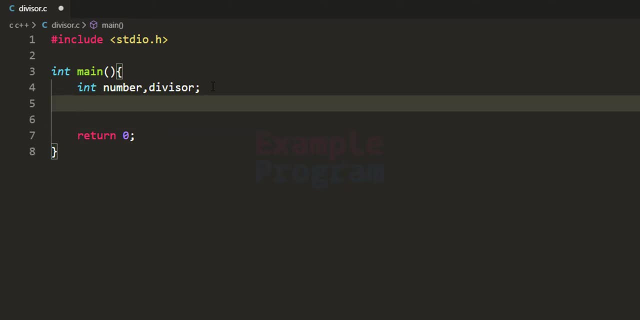 going to call it as divisor Now. the next thing that we need is for storing the divisor, So I'm going to call it as divisor Now. the next thing that we do is we will ask the user to enter the number. So I'm going to use a printf function in here and I'm going to specify the message as: 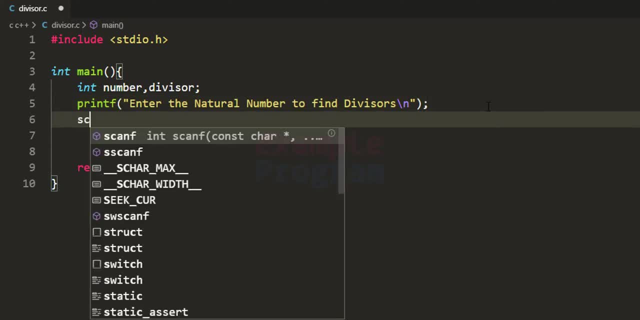 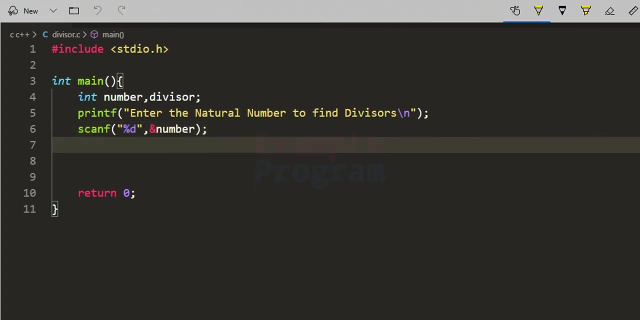 enter the natural number to find the divisors. and then we use the scanf function and here we will use the percentage d format specifier and whatever the number that we read, we will store that in this number variable. Let's say, the user is going to enter the. 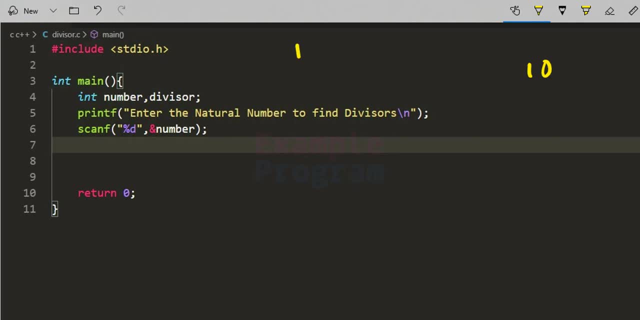 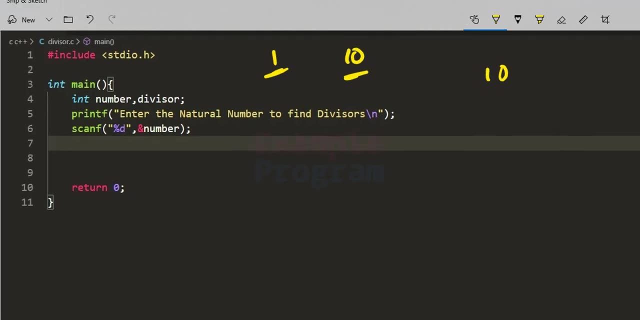 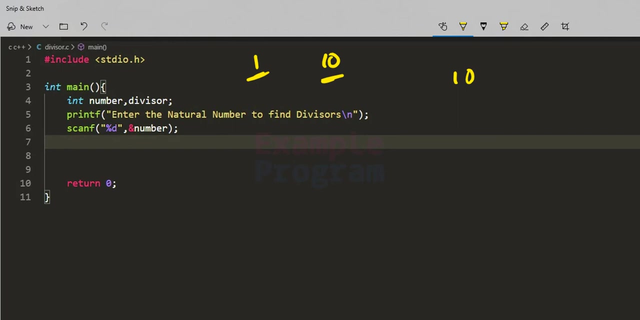 number 10.. Now we already know that the number 1 and the number itself, which is 10, these are the divisors of this number 10.. So since we already know this, we are not going to find it in our program. and then, if you look at this number 10, then the possible range of values which can divide: 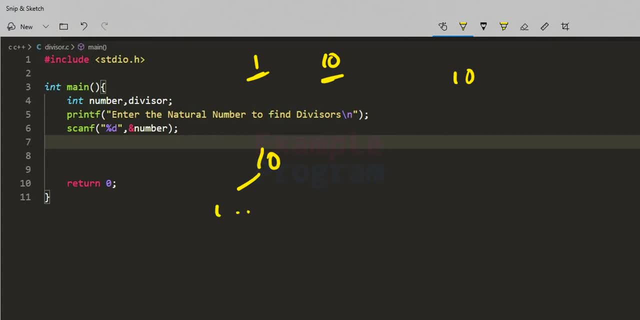 this number 10 completely are from 1 to 5.. We can say that the numbers 6,, 7,, 8,, 9,, 10 can't divide this number 10 completely and of course, 10 will do it. We already know this and we. 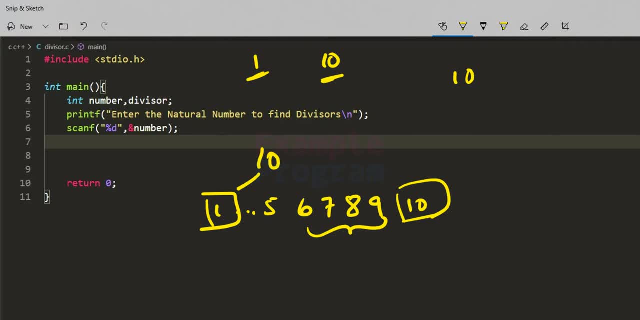 are not going to check for this number 1 and number 10 in our program. So the possible range of values are from 2 to 5 and in this range, this maximum value, 5, is actually half of this number 10.. So what we do is we take the number entered by the user in our program and we start dividing this. 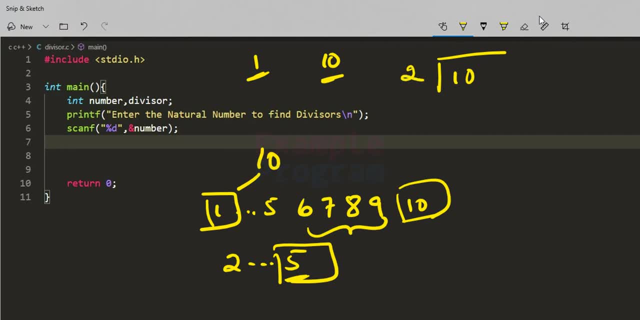 number, starting from the number 10.. So we take the number entered by the user in our program and we start dividing this number from 2.. So we will check the reminder value when we do that. If we get the reminder as 0, it means that 2 is the divisor of this number 10.. So we will display 2 and then 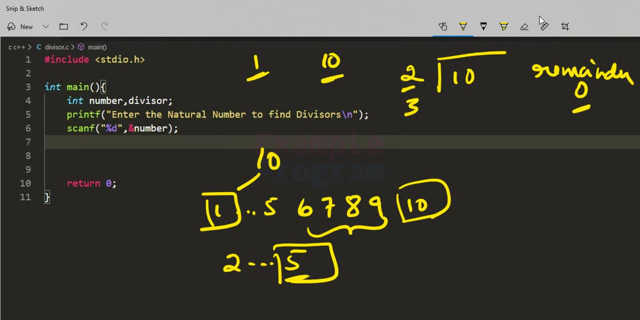 we go to the next number and again we will do the same thing. We will check for, we will divide it, We will check for the reminder value and we will display it. if it is the divisor, Then we will go to the next number and similarly, we go up to number divided by 2, because we are not going to 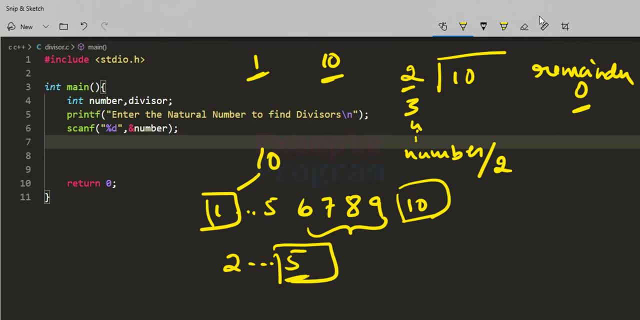 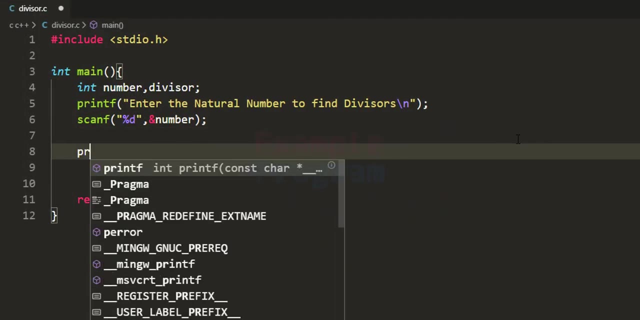 because, you know, these are the numbers which can divide, which can be the divisors of this number: 10.. Here, in this case, which is 5 number divided by 2, becomes 5, because the number that we are assuming is 10.. So, here, in this program, now let's use a printf function and we will say: 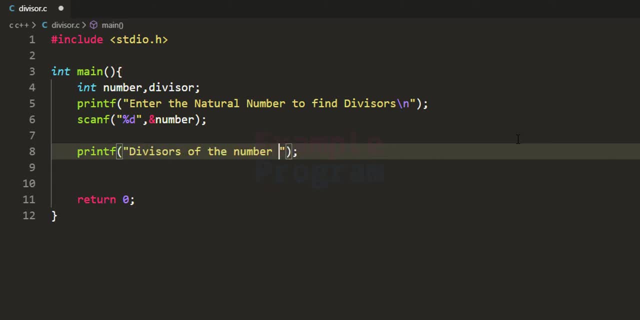 divisors of the number, percentage, d, r, and then we will insert this number variables value for the placeholder. and here what I'm going to do is I'm going to directly display the number 1 and the number itself. So I'm going to use a printf function. 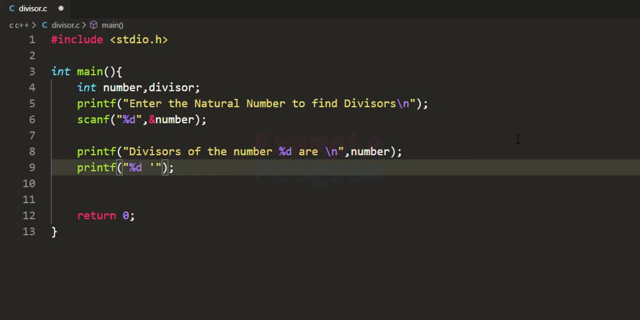 in here I'm going to write percentage d, space, percentage d- and then I'm going to add a space and here we will display 1 and the number itself. So after this we will use a for loop and in this for loop we will initialize our divisor variable with a value of 2.. That's because we 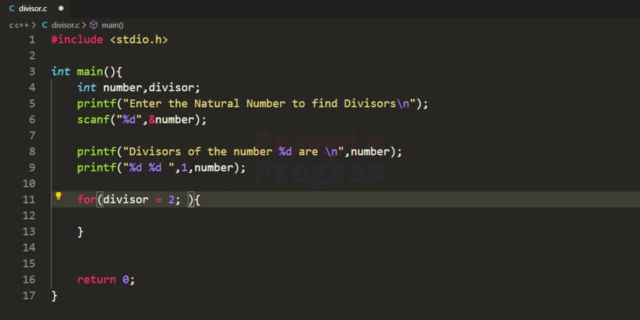 already know, 1 is the divisor, so we don't have to check for this number 1. and then the condition here will be: divisor containing a value less than or equal to number divided by 2, and after that we will increment the value of the divisor variable by 1.. So we will start from 2 and we will go up to. 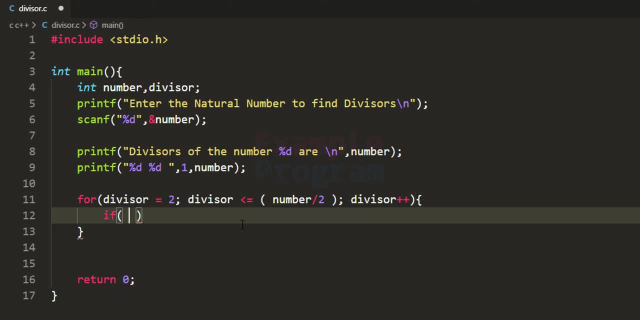 0, and here we will check what we get as the reminder value when we divide the value in the number variable by the value in the divisor variable, and here we will check for the reminder value whether it is 0 or not. This modulus operator returns the reminder value when we 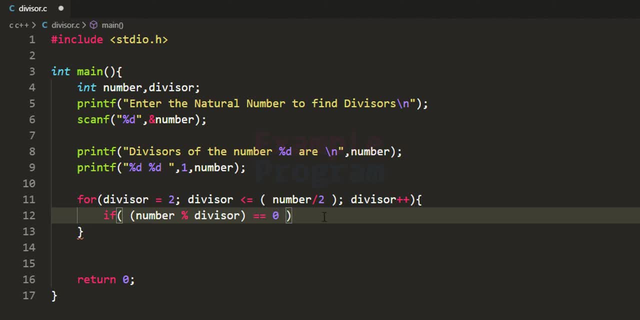 divide a number by another number. If we get the reminder as 0, it means that the value present in this divisor variable for that particular iteration in this for loop is the divisor of the number present in this number variable. So we will use a printf function and we will display that to the screen. So we will use 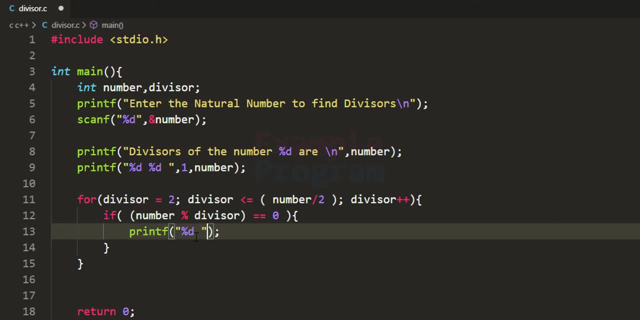 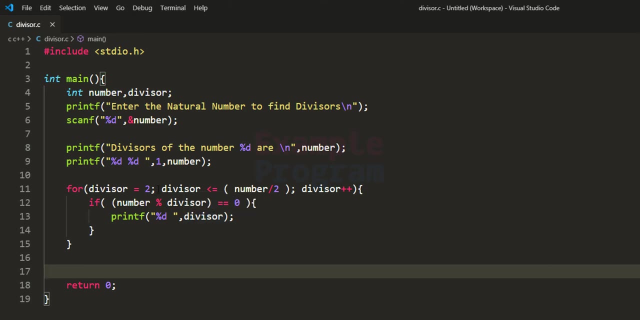 %d, and then we will add a space in here and we will display divisor variables value for that particular iteration. and if the reminder is a non-zero value then we are not going to do anything. So this for loop will start from 2 and it will run up to number divided by 2.. Now we have written the program, let's run this. 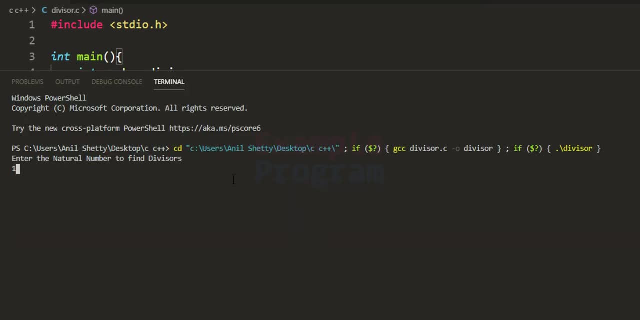 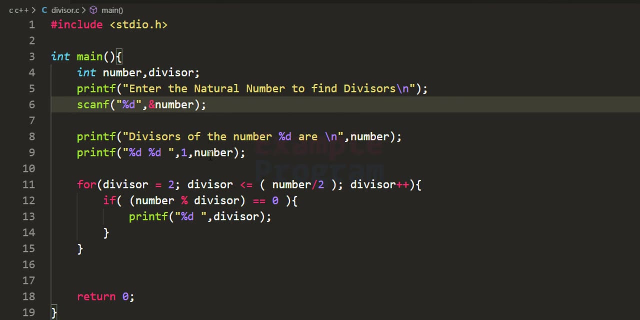 enter the natural number to find divisors. I'm going to say 10, it says 1, 10, 2 and 5, and here if you don't want to do it like this- you know you don't want to display the number 1 and the number itself like the way that I have done here- then you can modify this program. 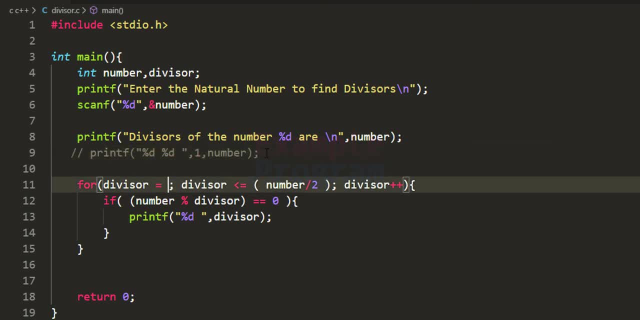 I'm going to come back to the program and I'm going to show you how to do it. So let's comment it out, and here we will make this divisor to start from 1 and we will change this condition to less than or equal to number. Now it will, you know, display the. it will check. 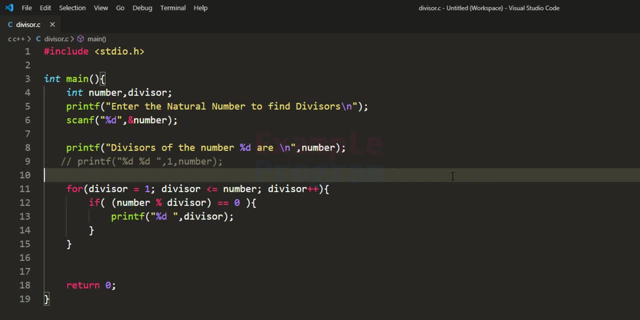 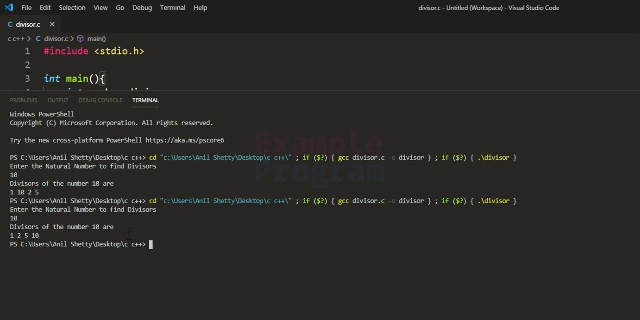 for the numbers starting from 1 up to the number itself. Now if I run this- and this time I'm going to enter 10, now you guys can see it will display 1, 2, 5 and 10.. So it will do a bit more calculation this time than it was doing in the previous run. 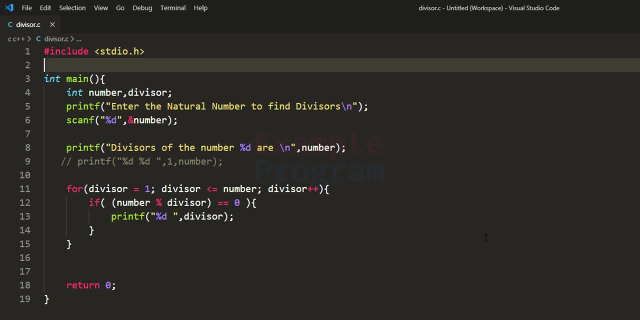 So this is it, guys, for this video. This is how you guys can write a simple C program to find the divisors of a natural number. If you like this video, then hit the like button. If you don't like it, then hit that dislike button. If you want to say something, then write that in the comment box. 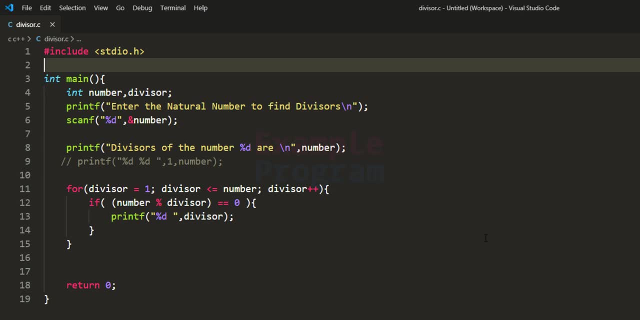 For more tutorials like this, do subscribe to the channel. Check out my website, exampleprogramcom, for the source code of this tutorial, and we also have a lot of programs in that website, Thank you. So this is it, guys. See you later in the next video.